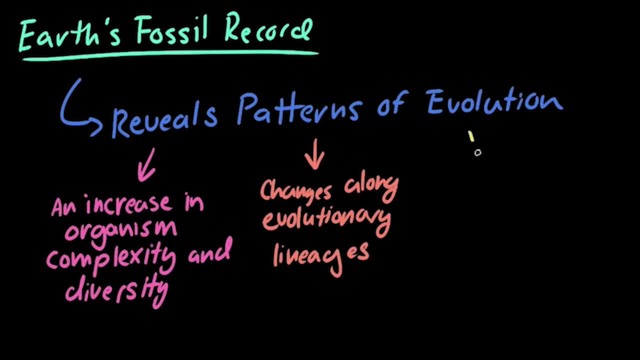 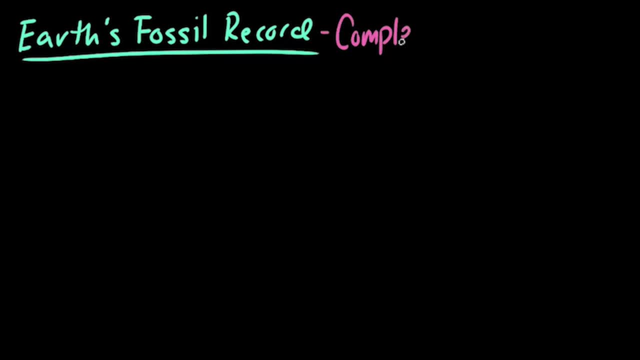 group of organisms could have evolved to the next. The fossil record also shows us when certain groups of organisms went extinct. First, let's take a look at the increase in organism complexity and diversity that is seen in the fossil record Over evolutionary time. 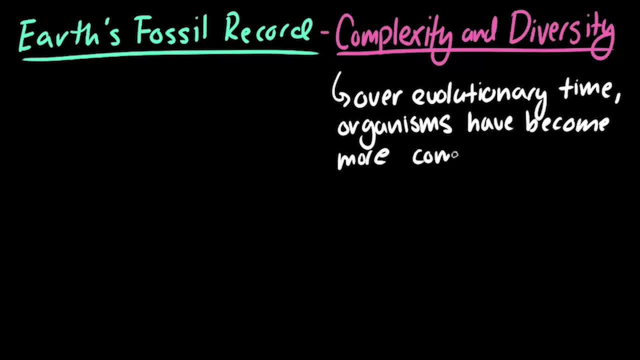 organisms have generally become more complicated. Some of the oldest known fossils are formations made by ancient colonies of cyanobacteria. These fossils provide evidence that single-celled organisms were living on Earth roughly around 3.5 billion years ago and that these organisms were 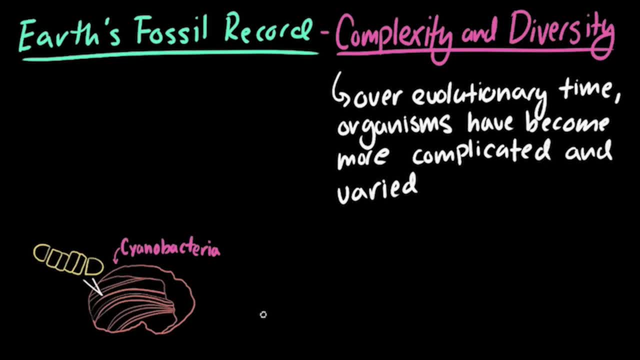 relatively simple, similar to the bacteria we have today. The fossil record then goes on to document major leaps in complexity of the life on Earth With, for example, the large, large tube-shaped cells of Grippania spiralis and the macroscopic organisms in the Francivilian. 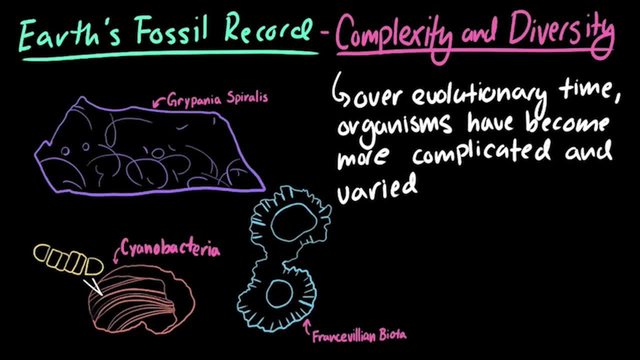 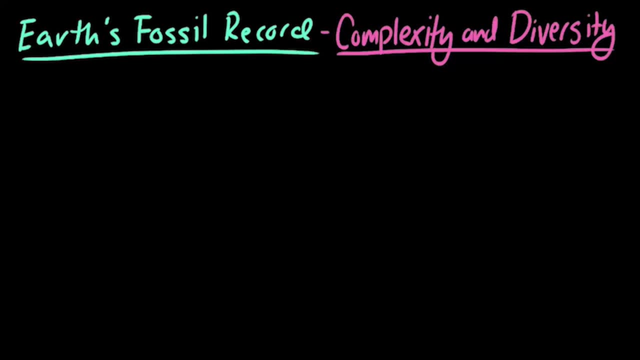 biota. According to scientists, these fossils, which are dated to be roughly from 2 billion years ago, could provide evidence of some of the earliest eukaryotic or nucleus-containing cells and of the earliest multicellular organisms. Not only does the fossil record show an increase in 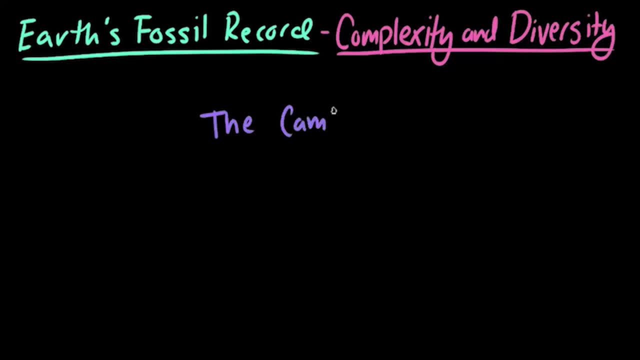 complexity over evolutionary time, but also an increase in the diversity of life on Earth. For example, the Cambrian Explosion describes a multi-million year span of time, beginning about 539 million years ago, in which there was a huge increase in the diversity of animals on Earth. 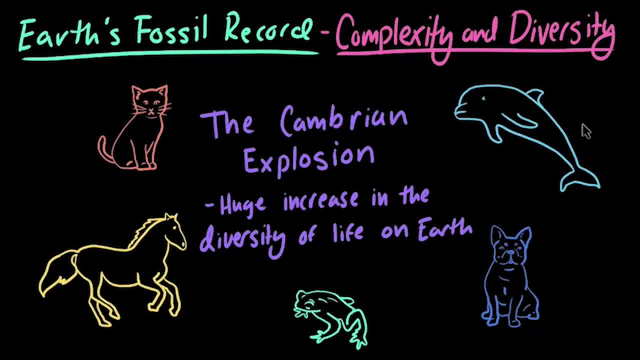 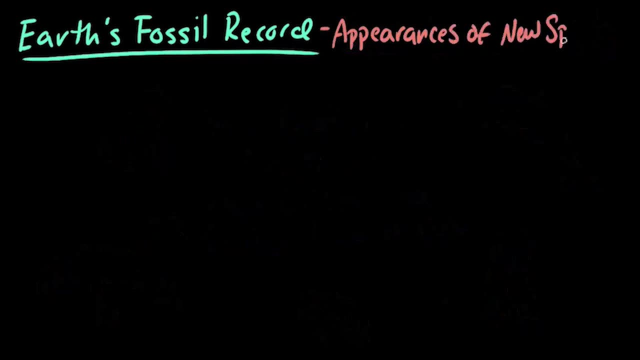 Almost all of the animal lineages we know today actually got started during this period. All of these increases in complexity and diversity have given rise to the millions of varied organisms that live on Earth today. Next, let's take a look at the changes that can be seen along the evolutionary lineages. 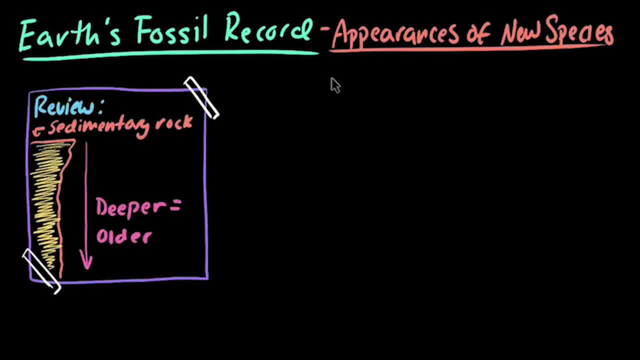 in the Earth's fossil record. But before we do that, let's quickly look back at how scientists study fossils. As you may recall, fossils are found in sedimentary rocks, meaning that the deeper the fossil, the older the fossil is likely to be. 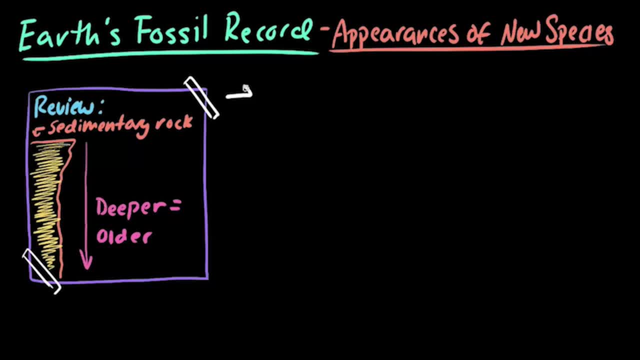 So, based on the layers in which the fossil is found, scientists can put them in order by age or by means of the ability of natural reactions, And in doing this, scientists can piece together the evolutionary steps of how one type of organism could have evolved into the next. 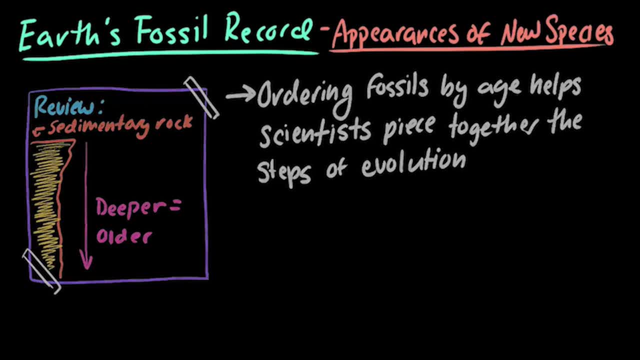 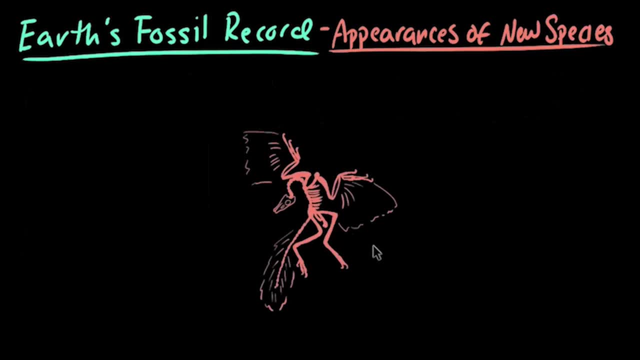 eventually giving rise to the living organisms we see today. To give an example of this, did you know that birds are actually direct descendants of a group of dinosaurs called theropods? It may be hard to believe, but the fossil record shows that an. 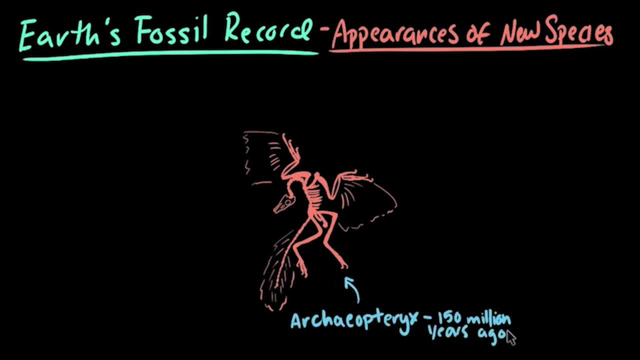 organism known as Archaeopteryx existed about 150 million years ago, towards the end of the dinosaur age, but before the appearance of modern birds. This organism in particular is interesting because it had some features unique to theropod dinosaurs, such as jaws and sharp teeth, and some features unique to birds, such as feathers. 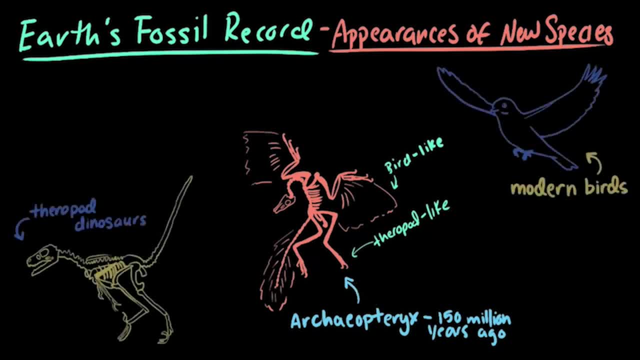 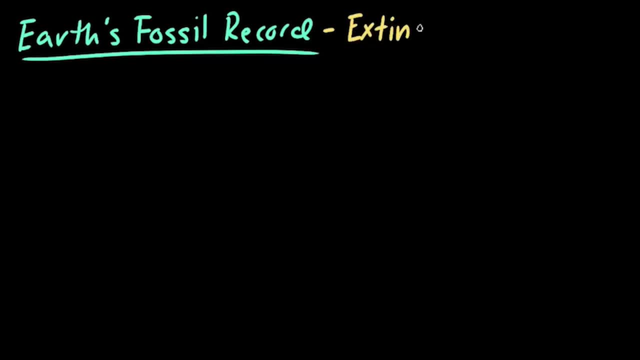 So Archaeopteryx represents an evolutionary transition between theropod, dinosaurs and birds in the fossil record. Finally, let's take a look at the patterns of extinction seen in the fossil record with the help of our extinct friend, the Triceratops. 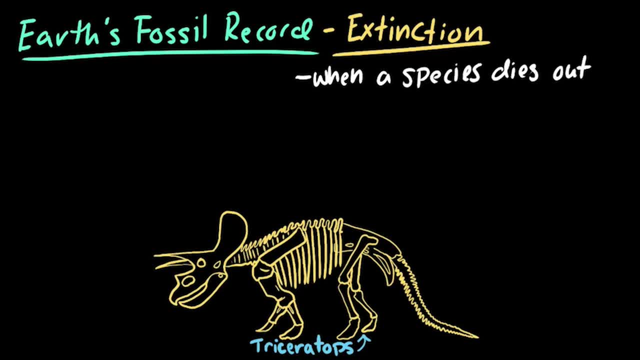 Extinction happens when a species completely dies out. In the fossil record, extinctions show up as organisms of a certain species being present in older rock layers and then completely disappearing from the newer rock layers. For example, we only see Triceratops fossils in rock layers that are roughly 68 to 66 million. 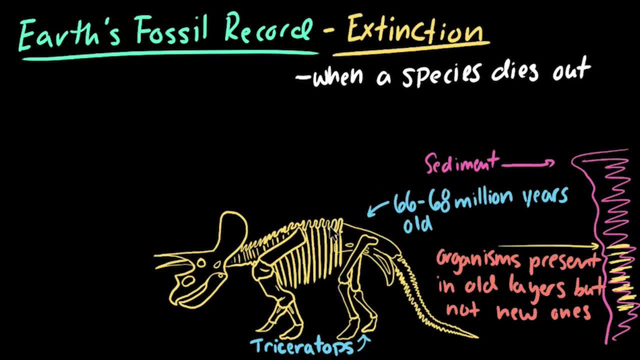 years old. After this, we don't find any evidence of Triceratops fossils, And there certainly aren't any Triceratops living today. The Triceratops is an important example of extinction, as they not only went extinct. 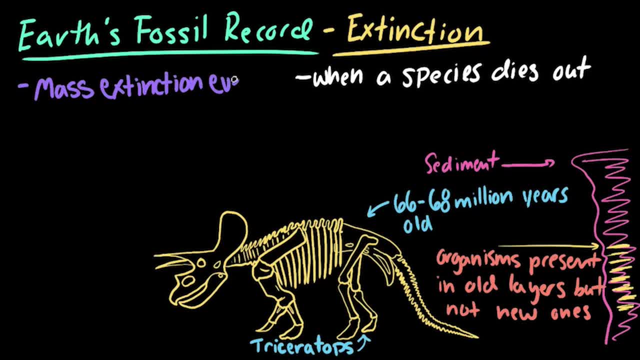 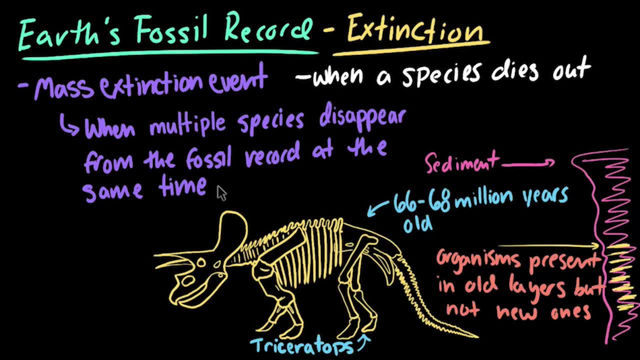 but they went extinct due to a mass extinction event. Mass extinction events happened when large-scale environmental change caused many groups of organisms to go extinct. around the same time, When we see the Triceratops disappear from the fossil record, we also see other types. 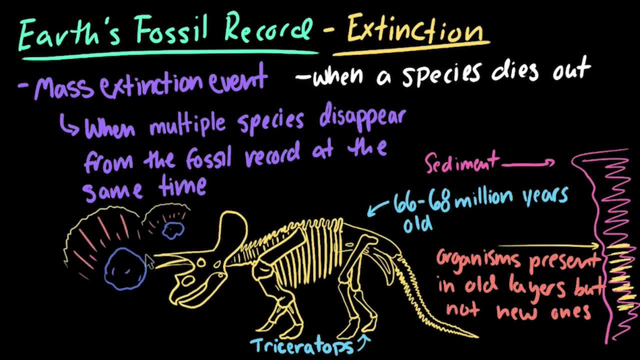 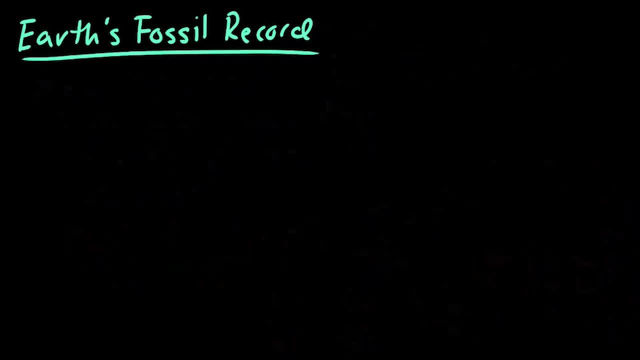 of organisms disappear too. Providing evidence: The Triceratops fossil record is a mass extinction event that led to the disappearance of all non-avian dinosaurs, And with that you now know what Earth's fossil record is and the various patterns it can. 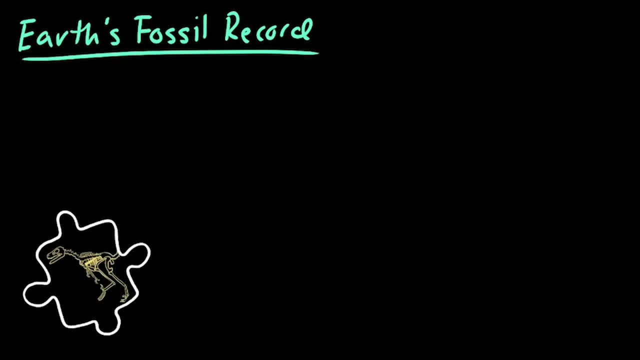 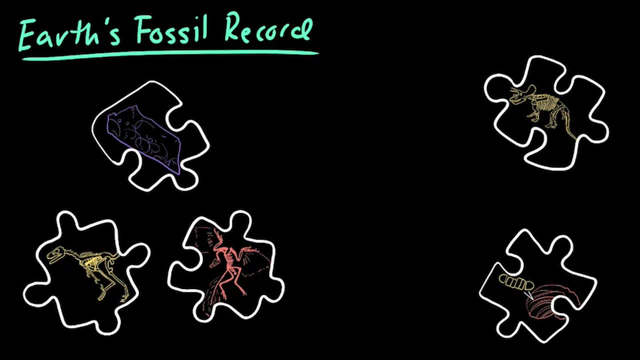 show us. Earth's fossil record is an essential tool that scientists use to piece together the history of life on Earth, And new fossils are continuously being discovered. So the fossil record is more than just a collection of fossils: It's a window into the mysteries of the past and its ever-growing record of how life on